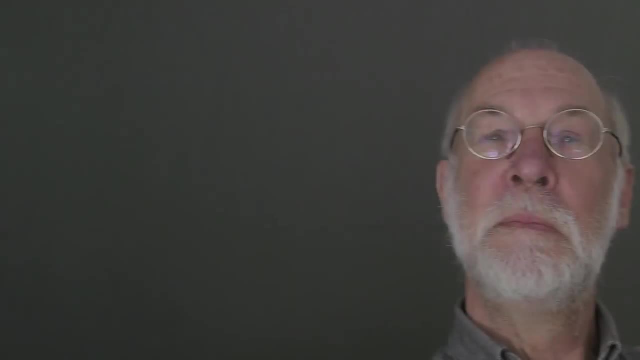 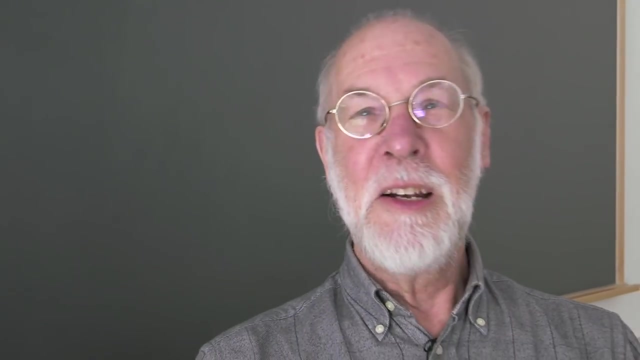 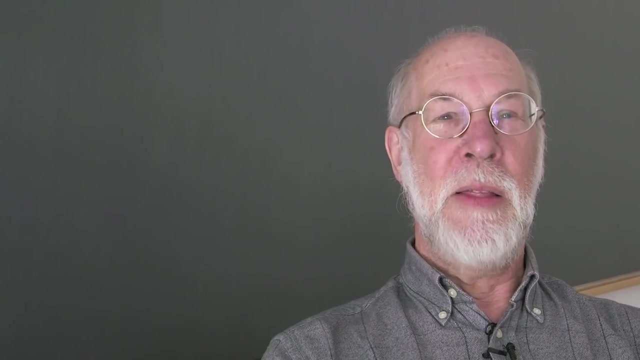 try it out like we did with these small primes. are we looking for a formula or like, a like a way to get those squares, or just no? impossible, that would be great. nobody knows a formula. you, you can only decide, if you have good luck, whether it is possible at all. not a formula which. 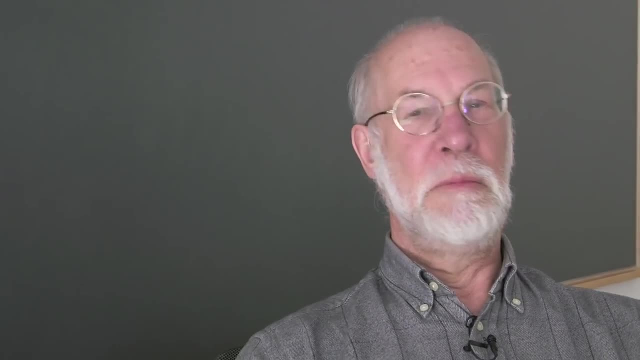 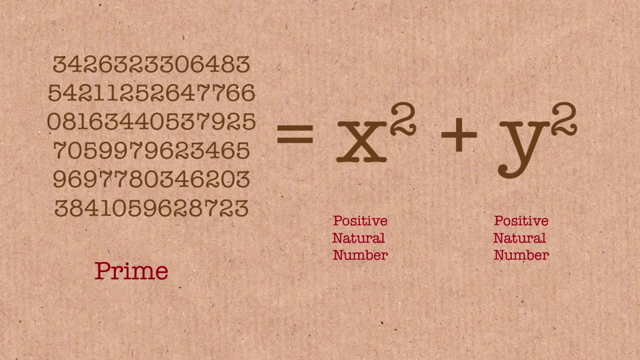 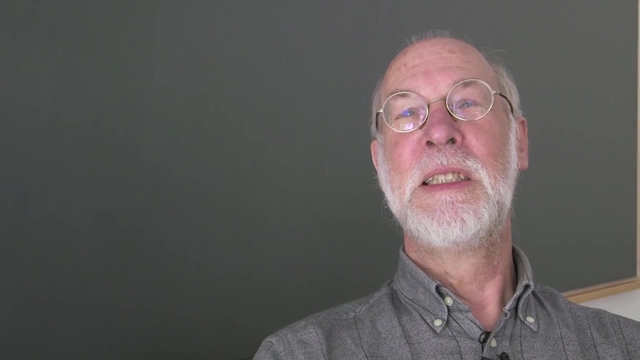 gives you X and Y. if you would give me some prime number. say, you search on the internet for large prime numbers, you give me one and tell professor: now tell me yes or no, and then in within a second I will tell you yes or no. but you won't. 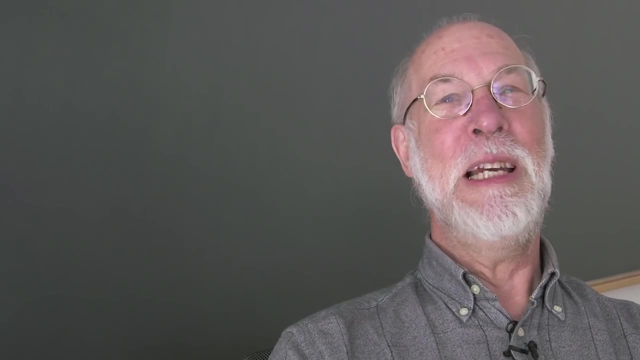 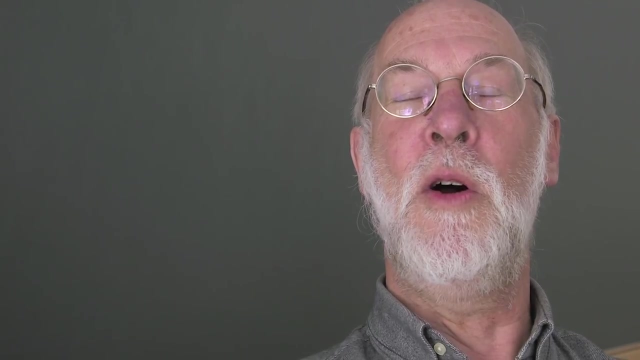 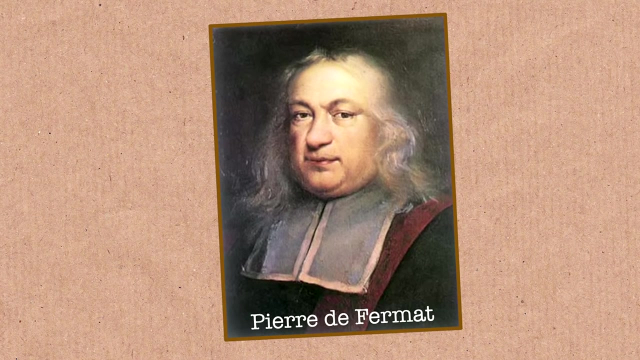 be able to tell me what those squares are? absolutely not. nobody will be able, not only me, I. just that we look into the history briefly. who did this first? this is the famous French mathematician, Pierre Fermat, who did other important things and he liked such easy to formulate problems. and what did he do with these? 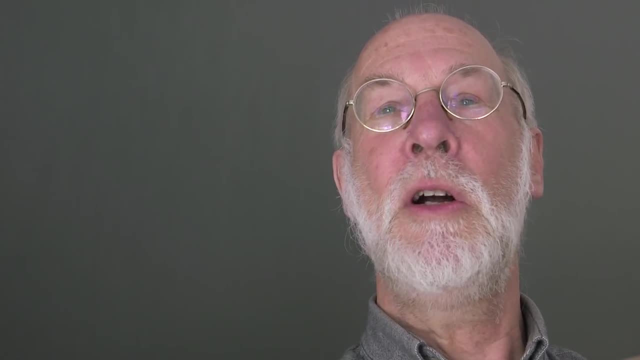 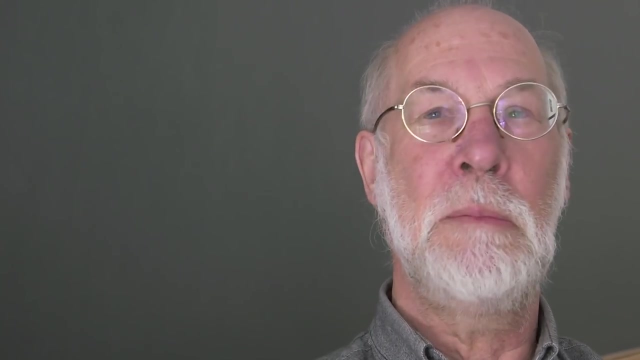 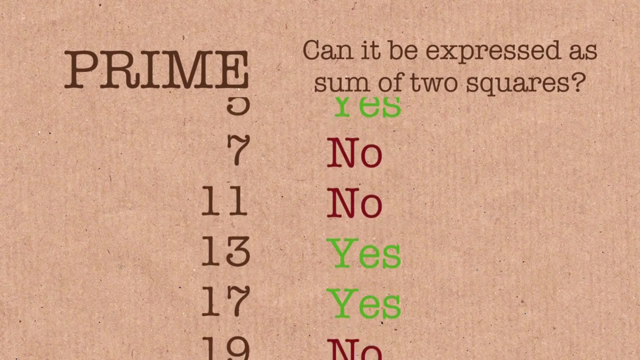 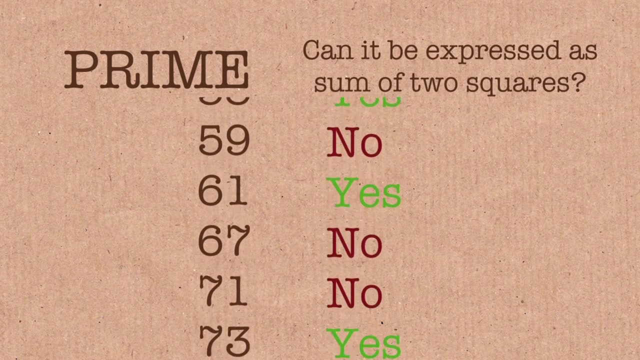 problems. he made tests. he made long tables so he took- we have here four primes. he took the primes up to hundred, the primes up to thousand. row down this list and checked by hand case-by-case. if you do that we can. you should show such a list. at the first glance you don't see any pattern. but 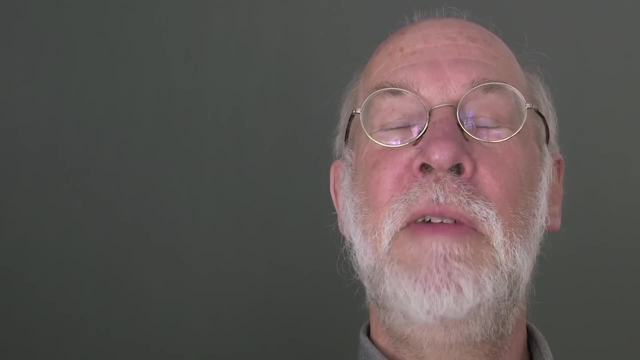 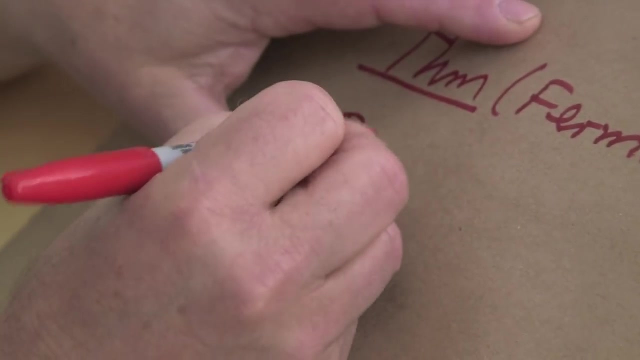 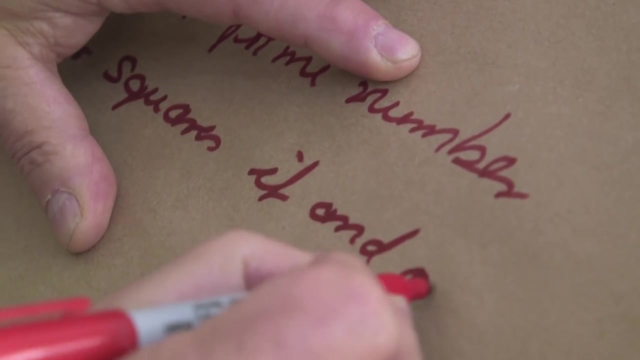 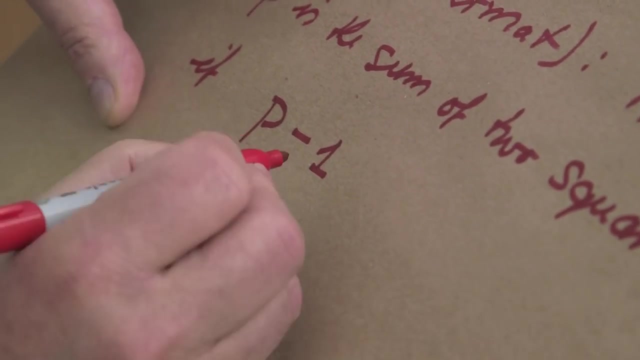 Fermat finally observed a very, very simple rule, and that's already his theorem, which I write down now: prime number P is the sum of two squares. if, I, If and only if we subtract 1 from p, we get a nice number if this number is divisible by 4.. 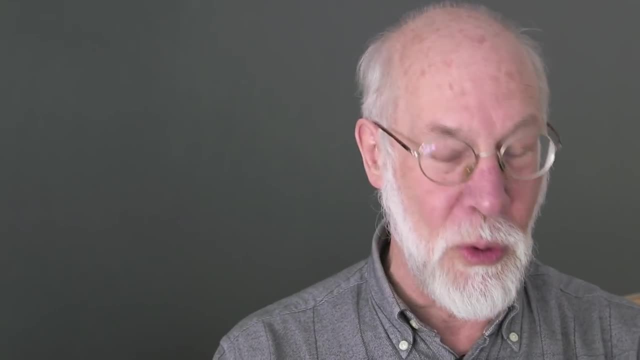 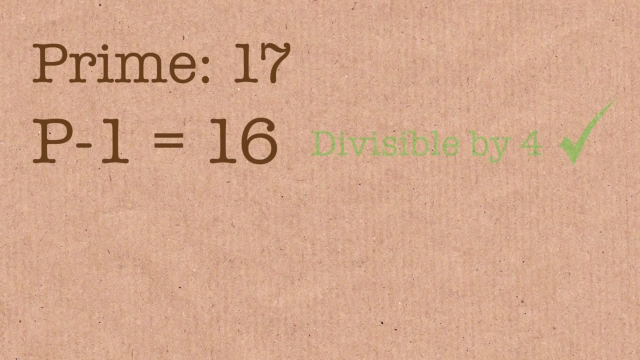 That means you can make a very, very simple test. So let's consider small prime. Let's say 17. We subtract 1,, we get 16. Ah divisible by 4. Ah, it works. And now we check. is it really true? 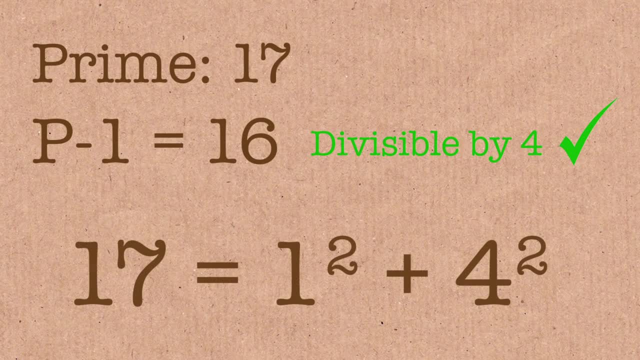 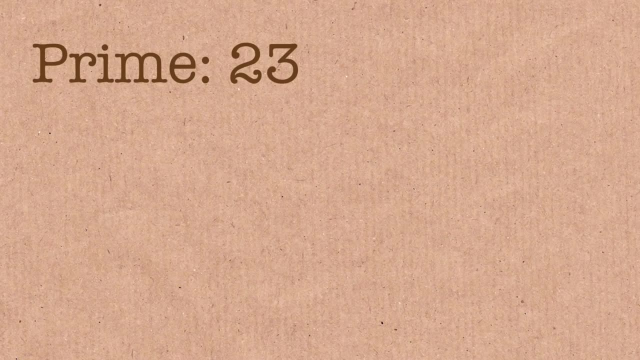 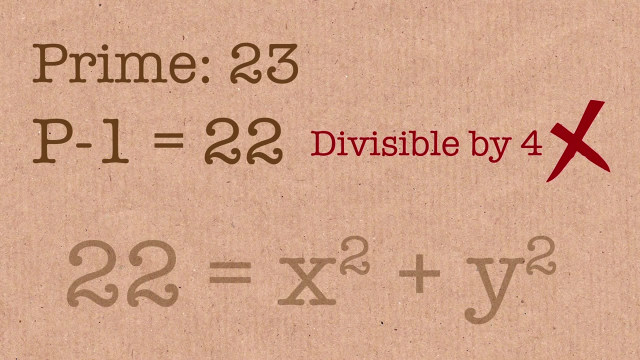 And we see: ah, 17 is 4 times 4 plus 1 times 1,. true, Let's consider 23,. other nice prime: We subtract 1,, get 22,, not divisible by 4.. So you can try it yourself at home. 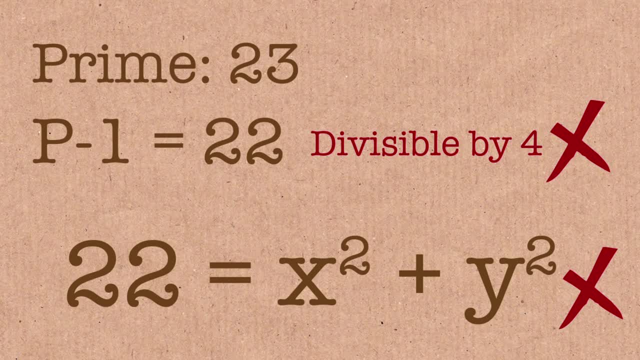 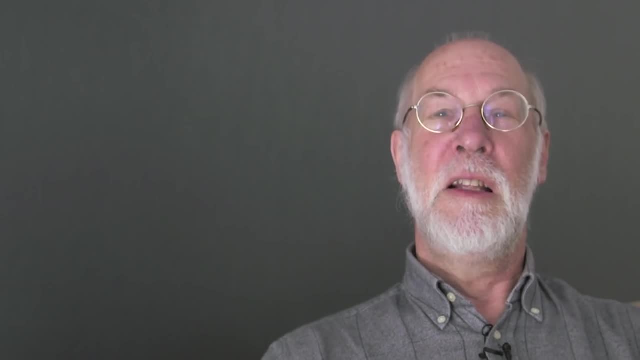 You will not be able to write it as the sum of two squares. The remarkable thing is this is an easy test to subtract and to check whether it's divisible. Divisible by 4 is very easy and you can try now on the internet. 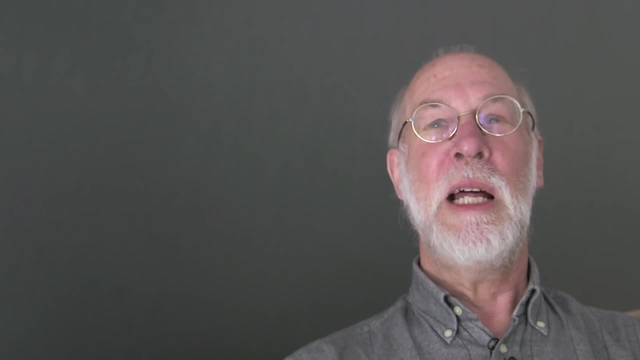 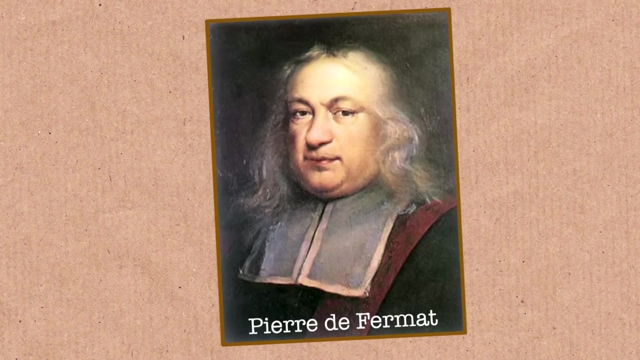 Write down huge prime numbers, subtract 1,, try to divide by 4, and you know here you go And you will not be able to find x and y. He saw it and he tested it again and again. We don't know whether he wrote down a proof. 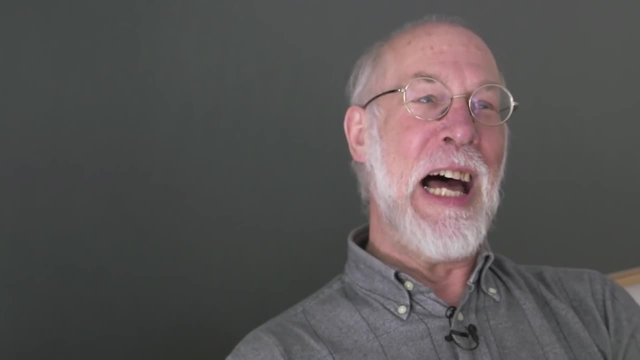 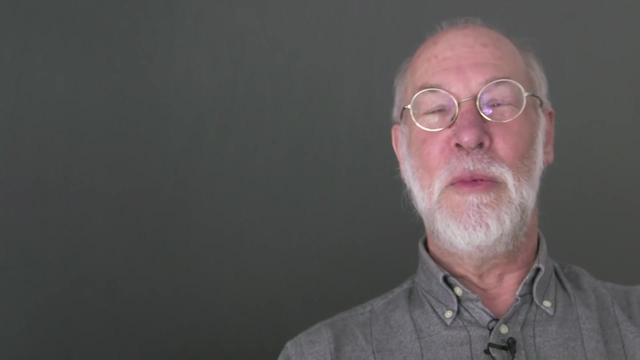 He said- it's a theorem, but he is famous for this He likes when he was convinced that something is true. he probably believed in God and in the order in the world. and he said: if I see this so often, it must be true. 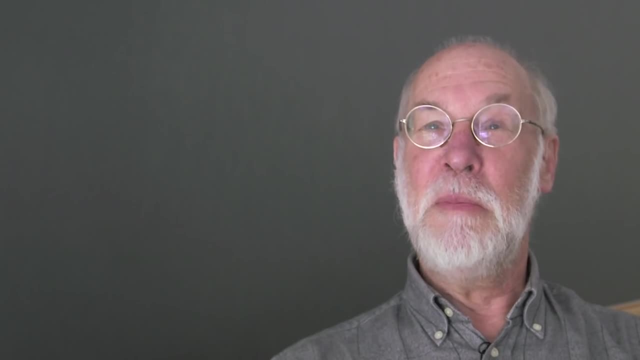 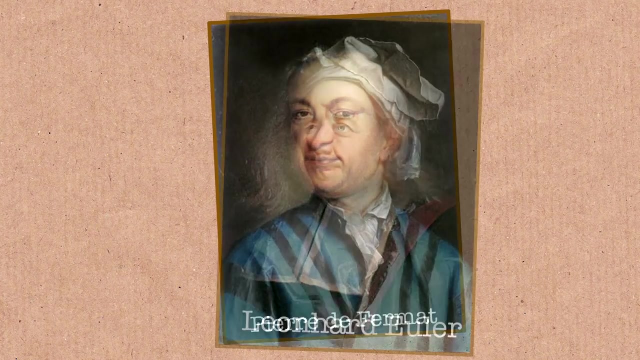 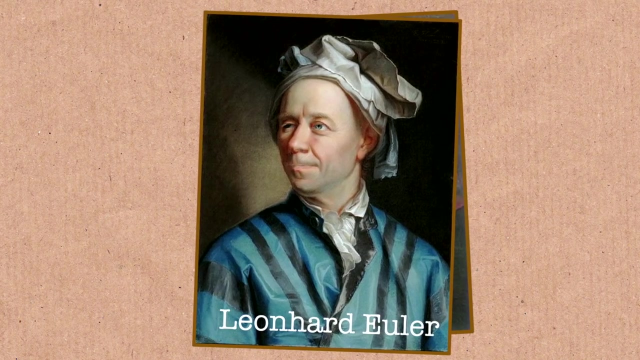 So he wrote down a theorem, but without proof, And the mathematicians after him wondered about the proof- Very good mathematicians- and could not do it. 100 years later, the Swiss mathematician Euler gave the first proof: A tricky proof, Complicated, Too complicated for this video. 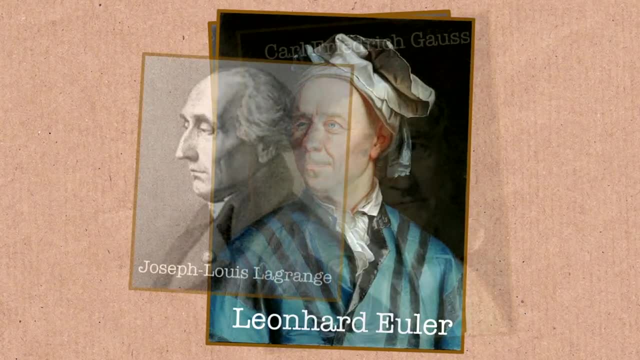 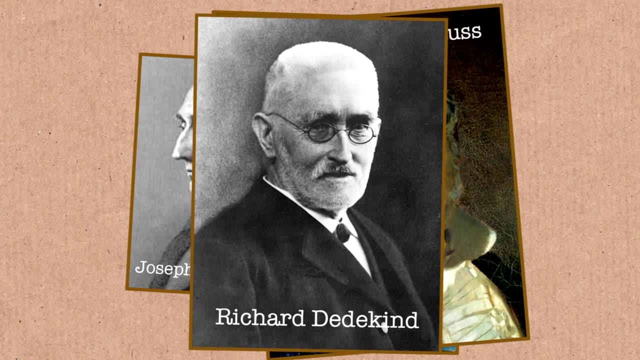 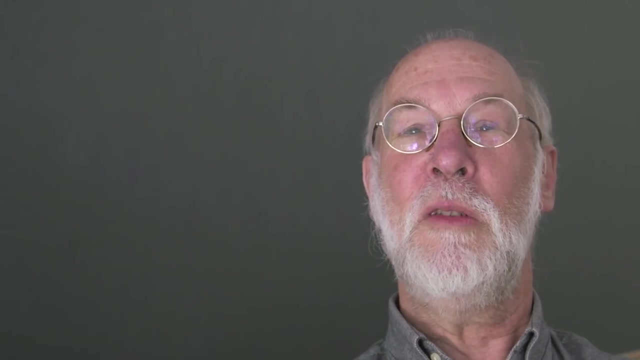 First proof. Then, 50 years later, Gauss gave a completely different proof. 70 years later, Didekind gave again a completely different proof. So the mathematicians like to give different proofs of the same theorem, because of every proof sheds light on the statement. 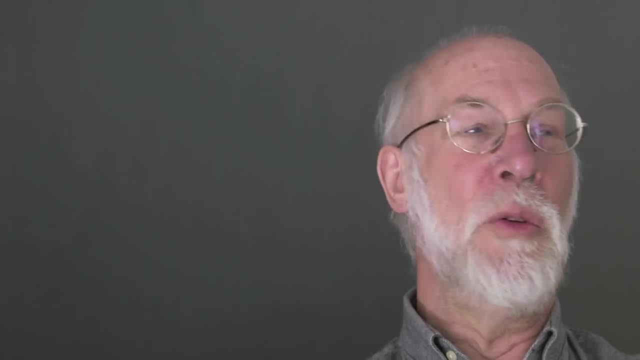 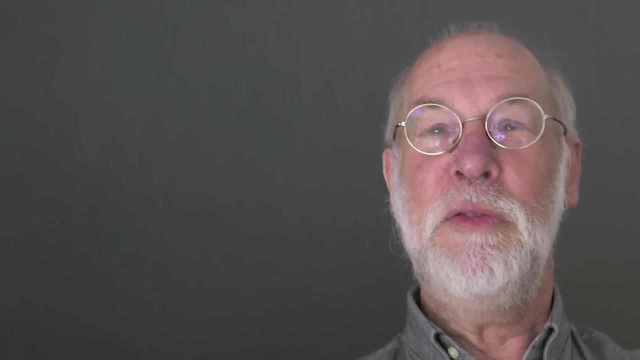 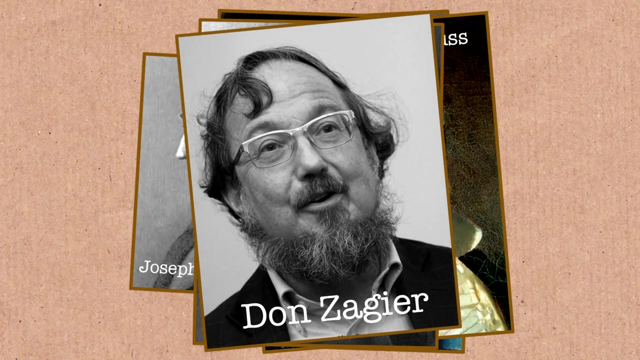 And all these proofs shed different light on the statement. So that's all. these proofs are too complicated even to speak about that here, But about 50 years ago the mathematician Don Zagier from Bonn gave the famous one-sentence proof. 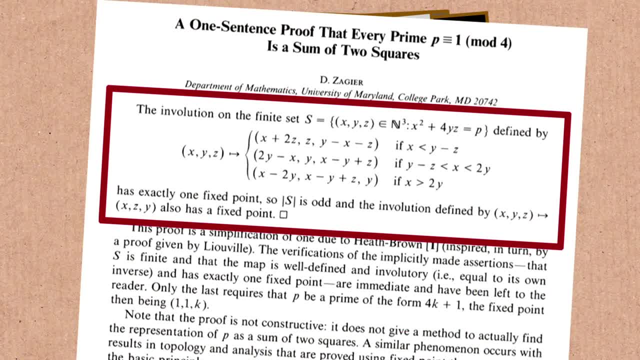 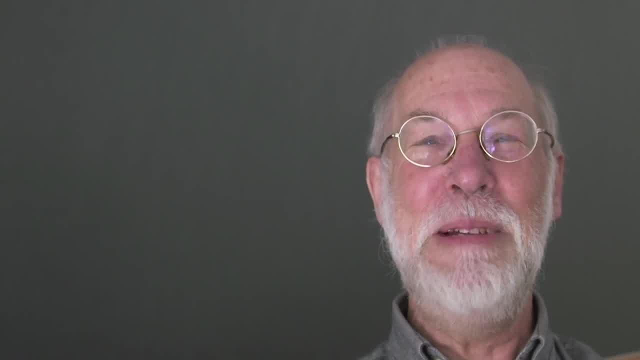 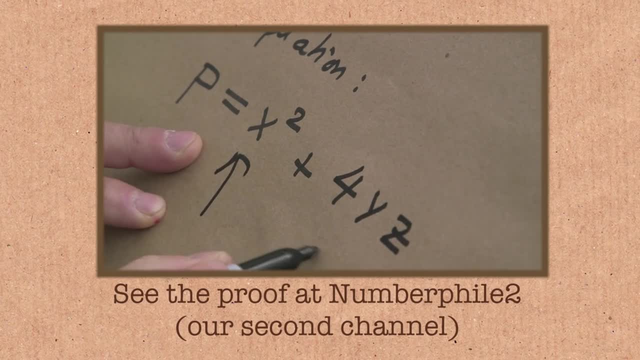 And that we are going to talk about One sentence In one sentence. Of course, you will see, for an ingenious mathematician like Zagier, it can be done in one sentence. For ordinary mathematicians like me, I need already ten sentences.